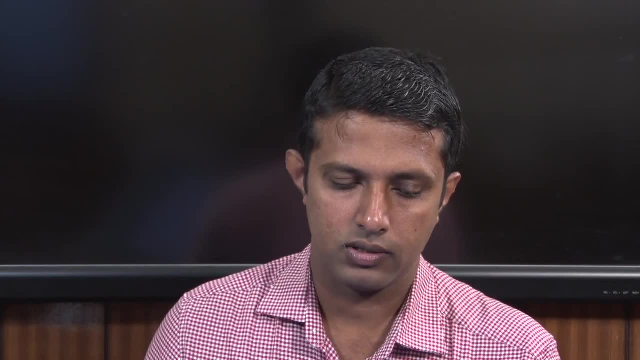 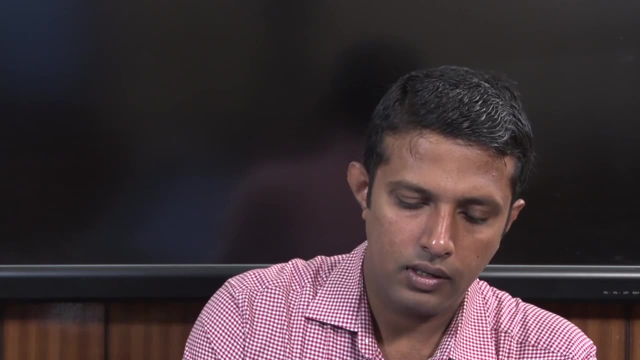 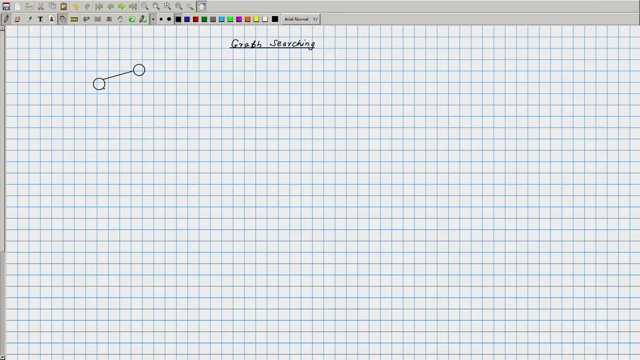 certain node and you want to know all your connections. So you want to know who your friends are, their friends and so on. So you can think of this as a huge graph in which each person is a node and there is an edge between two people if they are friends. So 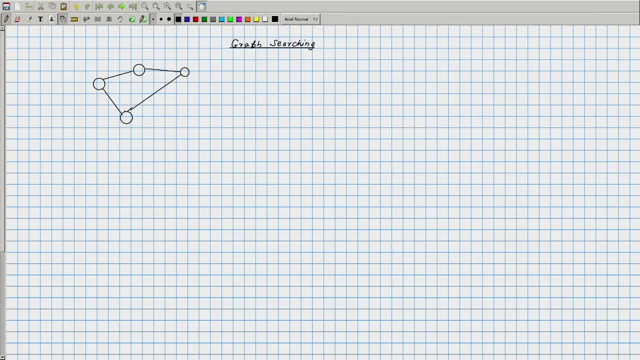 you have given some such graph. So here there is an example of 4 people: 1,, 2,, 3 and 4, and here 2 and 4 are friends with each other and they are friends with one as well. ok, 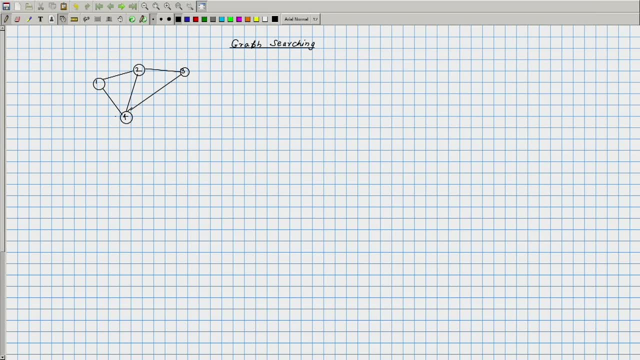 So you are given some arbitrary graph. How do you look at all the vertices, list all the vertices in a certain order, restricted to, let us say. I mean, if you think about the case of social networking sites, you want to order all your connections in some order. ok, 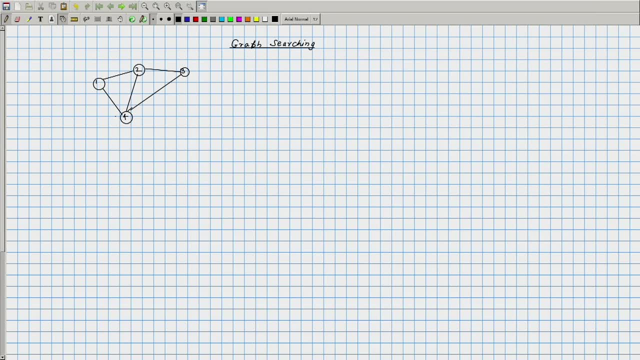 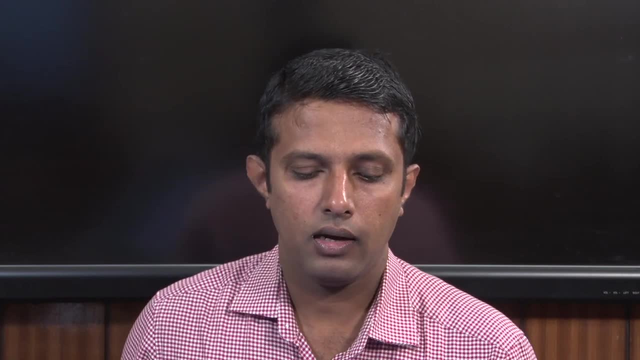 You can either look at, I mean you can look at your friends, List them all of your connectors. Just lock the 32 Steps Toある sailor. You can list, because they cannot work as one node is another. Its institutions may are Monte out and then friends of friends, and then friends of friends of friends, and so on, and that would 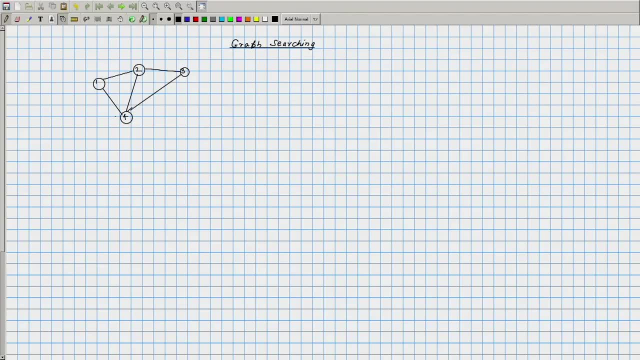 essentially be what we will refer to as breadth first search. You can also look at an alternate approach. you find one of your friends, look at another friend of his and keep on doing that sequence of friends. then you will get what is called as DFS. okay, 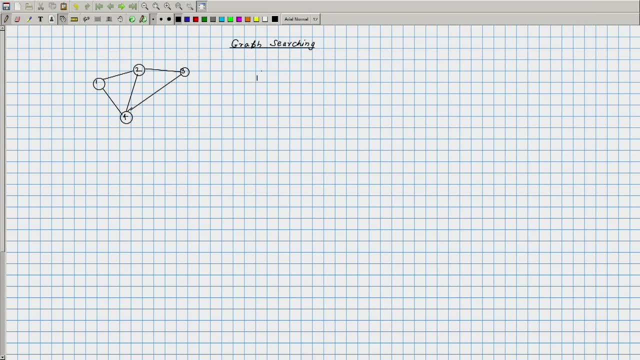 The commonly used searching techniques. we will just write them down: breadth first search and depth first search. So here, if you start your search at vertex 1, we may view vertices 2 and 4 are the vertices at depth 1 and the vertex 3 is at depth 2.. 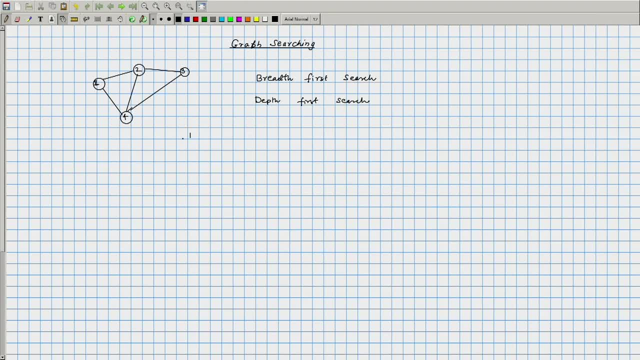 Okay. So if you look out at the order, 1, followed by 2, 4 and followed by 3, that would be the breadth first search. You have listed them in the order of their depths. that is called as a breadth first search, whereas if you list it as 1,, 2,, 3, 4.. 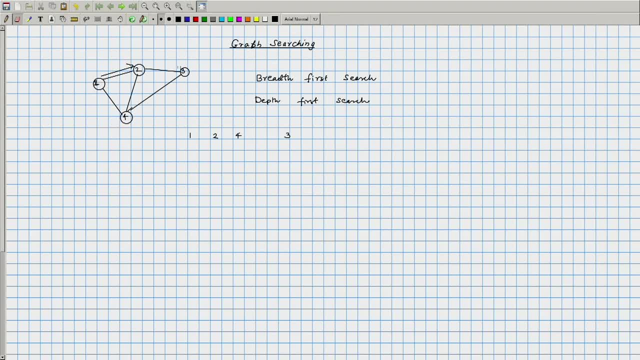 So you have gone from 1 to 2, from 2 you could go to 4, from 4 you could go to 3.. Okay, But there are examples where these two searches return different orderings. Okay, So let us look at this more formally. let us first look at a little more complicated. 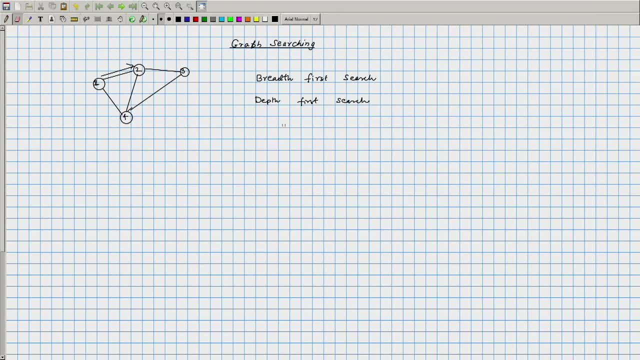 example. So we have the following graph: Okay, Suppose we have this graph, what will the BFS ordering be and what will the depth first search ordering be? Okay, So we will first write down the BFS ordering, starting at vertex 1.. So the start vertex, let us color it using red. this is just to indicate that it is a. 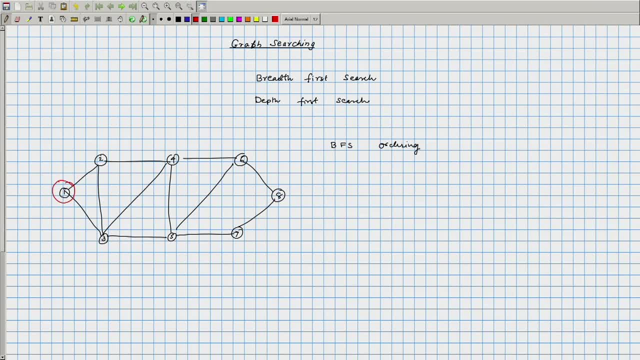 starting vertex. Okay, So that will be the first vertex that is encountered in BFS or in DFS. and now look at all the neighbors of 1, there are precisely 2 neighbors, 2 and 3, list them out, you will get 2 and 3.. 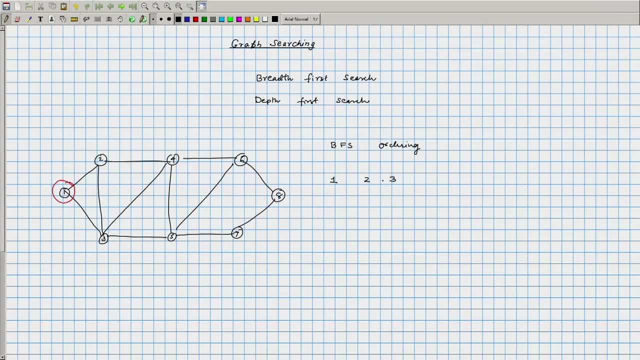 Okay, And the next stage would be to list out all the neighbors of 1.. So we will list out all the neighbors of 2, followed by all the neighbors of 3.. We do that in this case, the neighbors of 2. there is 3, so we will not list out the already. 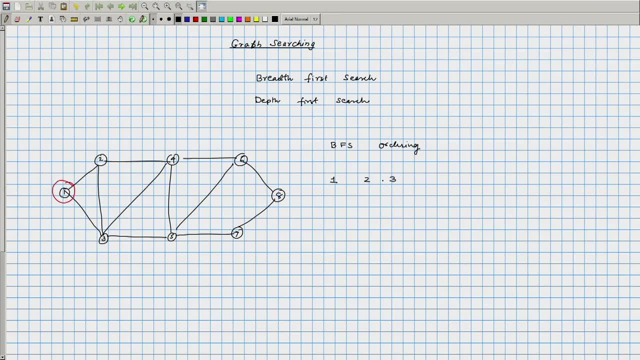 listed neighbors. So there are precisely 2 neighbors, namely 4 and 5.. Okay, So 4 is a neighbor of 2 as well as 3,. 5 is a neighbor only of 3 and not of 2.. Okay, 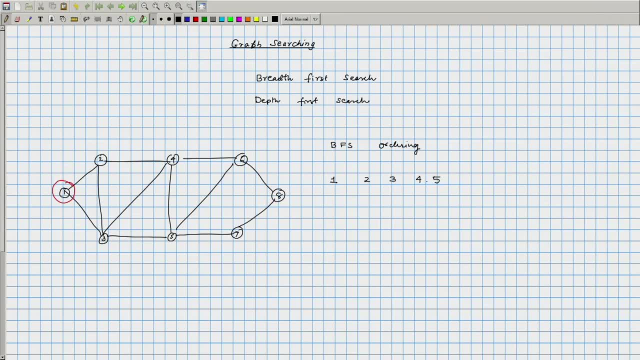 And then we will list out neighbors of 4 and 5, and we will get 6,, 7, and then we have the neighbor 8.. Okay, So this would be the BFS ordering, whereas if you take the DFS ordering, so let us say: 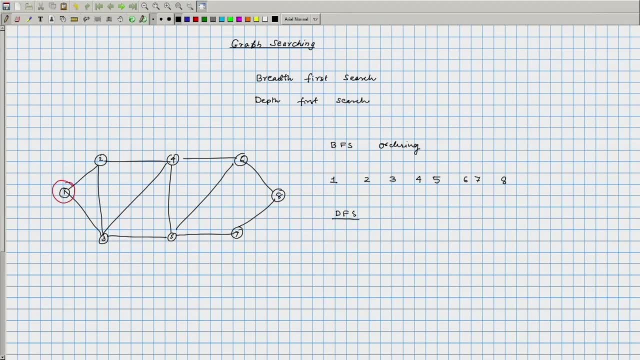 so in BFS ordering it is not a. I mean it is not fully determined in the sense the did we vertex visit vertex 2 before 3 or do we visit 3 before 2? that is not really specified. you could visit in any order and that has a chain of other choices that may not be fully. 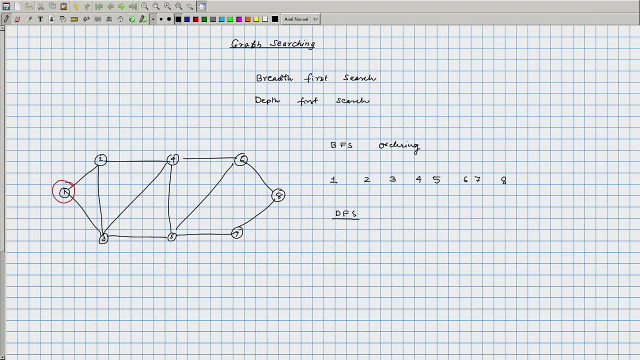 determined. Okay, The same applies in DFS. which neighbor you pick, there is no restrictions in either BFS or DFS. But whether you look at all neighbors, Okay, Look at all neighbors of a node and then go to the next level, or whether you keep on traversing. 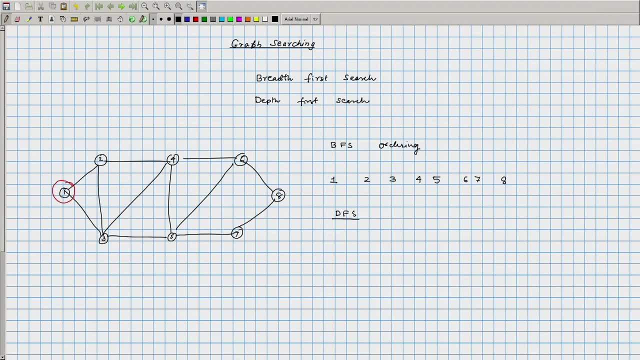 the graph, layer by layer, from one vertex to its neighbor and then to its neighbor, and so on. So that is what differentiates BFS and DFS. Okay, So DFS ordering from. so you could go from vertex 1 to vertex, let us say 3, and from 3,. 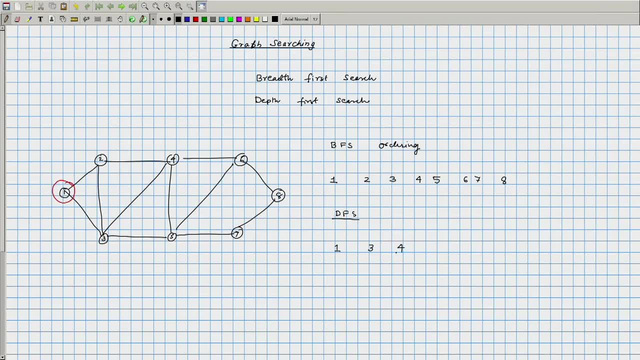 you could go to 4, from 4 you could go either to 5 or 6.. So the ones which we have visited, we will just draw in red. So 1 to 3 we went, and from 3 to 4 we went, and then 4 to 6 we could go, and from 6 we 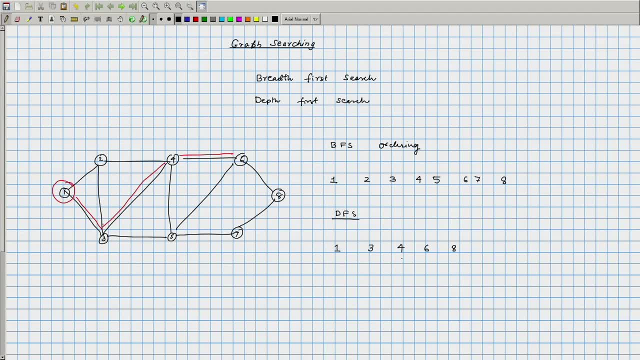 could go to 8, and from 8 we could go to 7.. Okay So, that is what differentiates BFS. Okay So, from 7 and from 7 we could go to 5, and after we have reached 5, we see that all its. 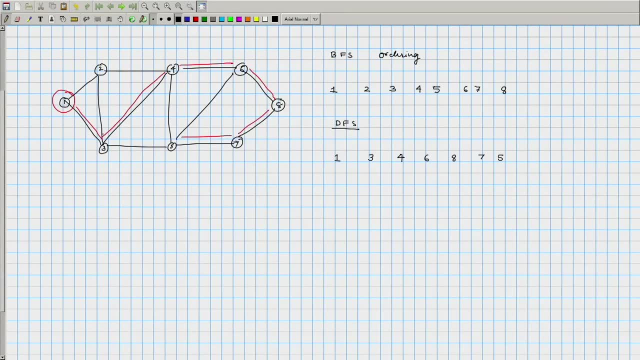 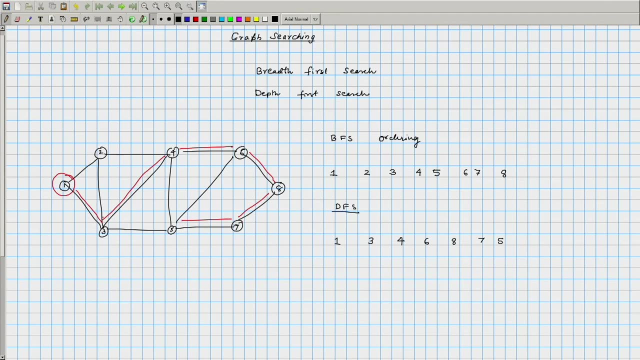 neighbors are essentially visited. okay, So the neighbors of 5 are 3,, 4 and 7.. So the neighbors of 5 are 3,, 4 and 6. All of them are visited. So you go back to the node from where you came to 5, namely 7.. 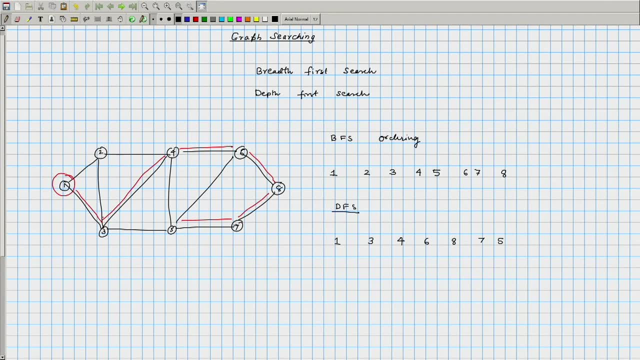 Its neighbors are all being taken care of, Same with 8,, same with 6,, same with 4.. You backtrack all the way up to vertex 4.. 4 has a neighbor which is not yet visited. So that is node number 2.. 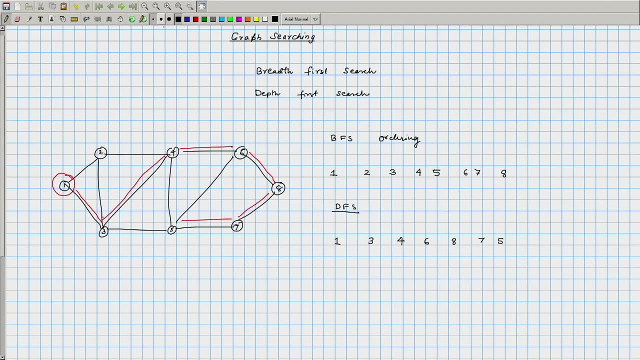 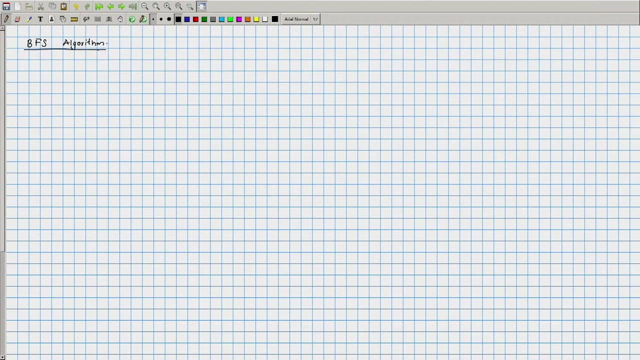 So that will be the last node that is visited. okay, So this will be the DFS ordering. Okay, Okay, So now we will see how we can algorithmically implement this. We will see an algorithm for BFS doing these searches. What we will do is the following: 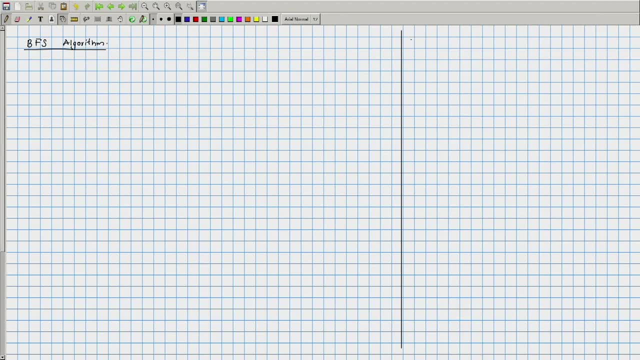 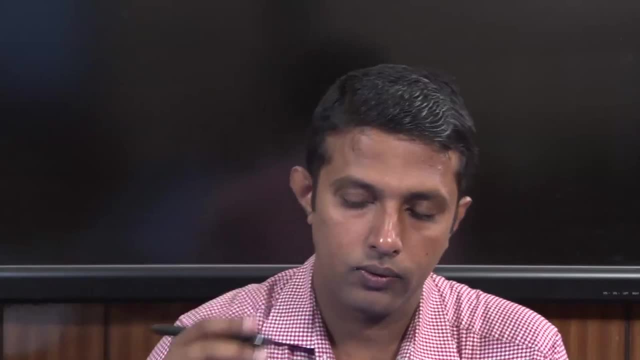 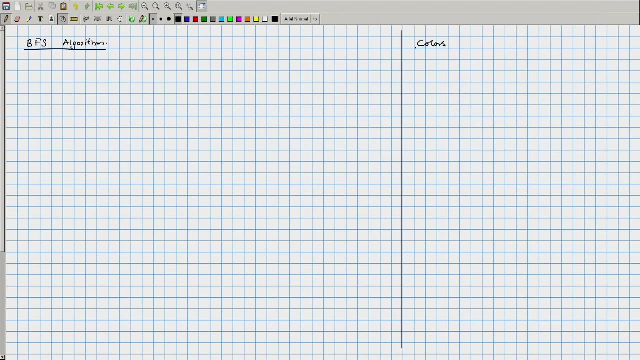 We will have colors associated with every vertex. These colors is to indicate whether certain vertex has been visited, whether all its neighbors' have been explored, and so on. Okay, So we will have 3 colors. So colors will be one attribute. Another attribute would be its predecessor. 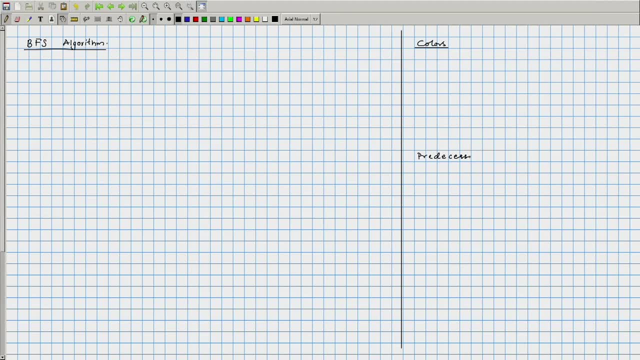 Each vertex will have a predecessor, So this will indicate the vertex from which we explored the given vertex. So if you have a vertex u, So u dot color will initially be white. Okay, For every vertex. So this is the start state. 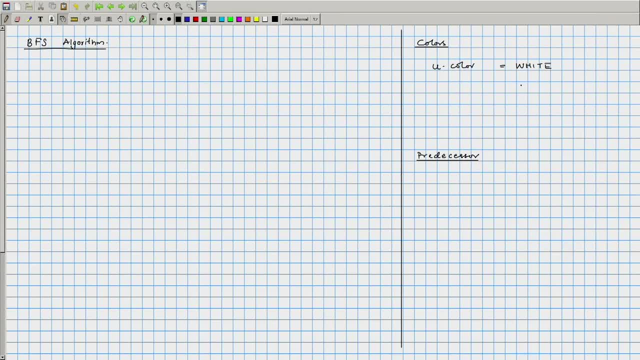 Every vertex will be initially white. The other colors are gray and black. Gray would mean we have partially explored that vertex and it is still under process. Some of its neighbors have been explored, Some of them have not been, and black basically means all its that vertex, everything that. 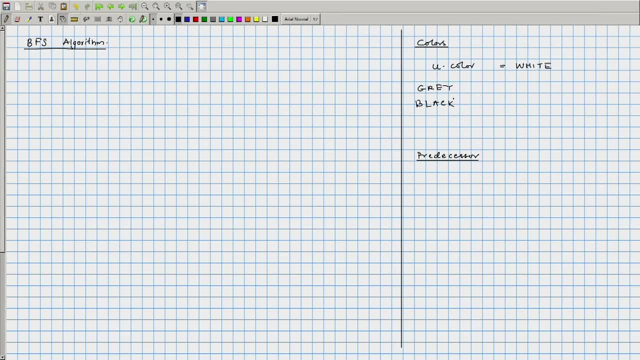 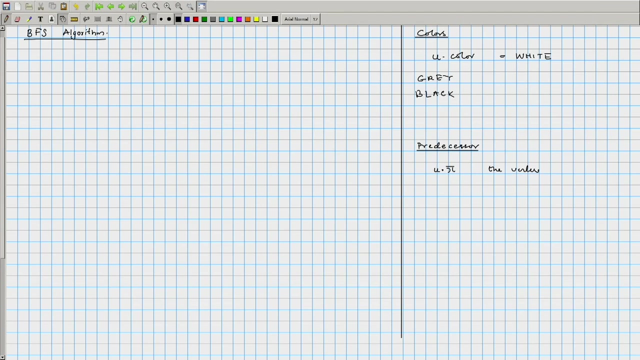 we have to do with respect to that vertex is over. We have finished the processing of that particular vertex And there will be another parameter associated with each vertex that will be its predecessor. So we will denote it by u dot pi. So u dot pi would mean the predecessor of u, and this is the vertex from which we have. 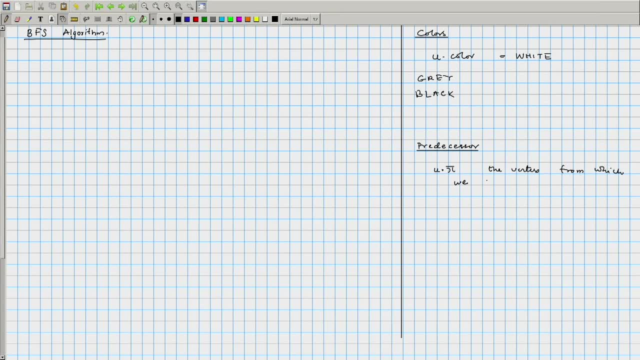 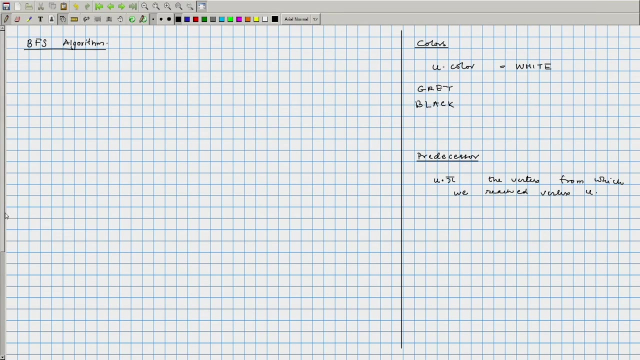 the vertex Okay. Okay, So we have reached vertex u, So that will be the predecessor of u. Okay, Now our algorithm. the way it works is it will have a q and we will push these vertices into a q as the algorithm progresses and after the all processing is done, we would 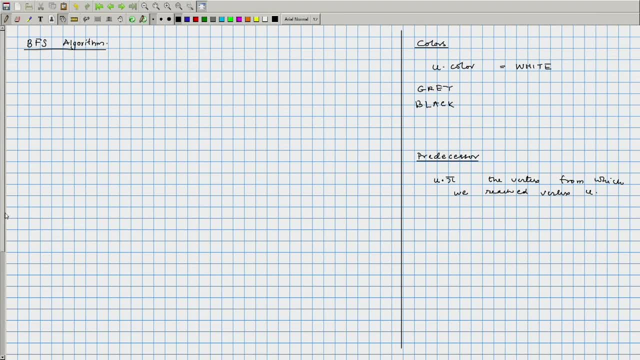 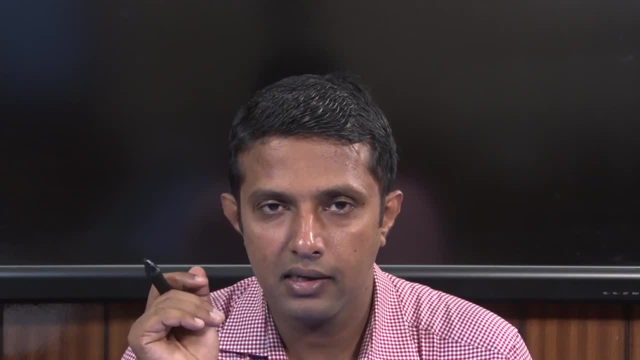 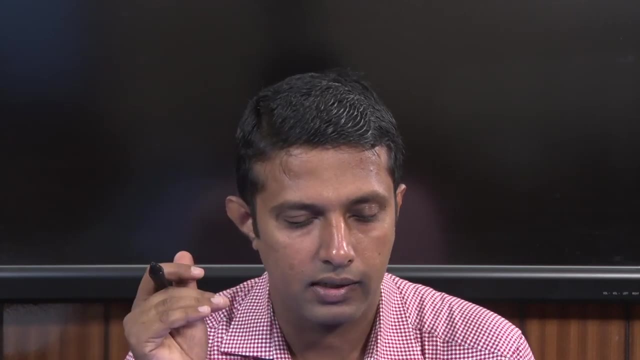 have visited all the vertices from a given static point. Okay, Okay, So we have a given starting vertex. We will assume that the initial graph that is given to us is an undirected graph, which is a connected graph. Of course, BFS would work even if the graph was a directed graph and if it was a disconnected. 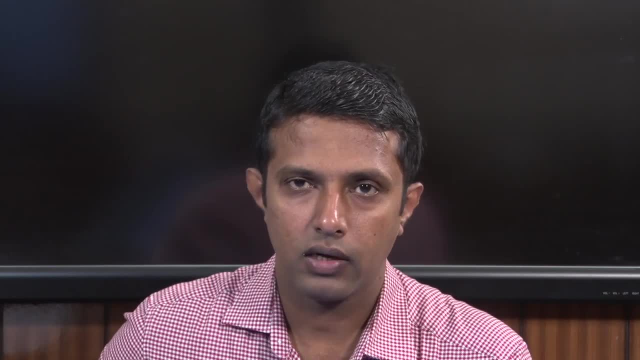 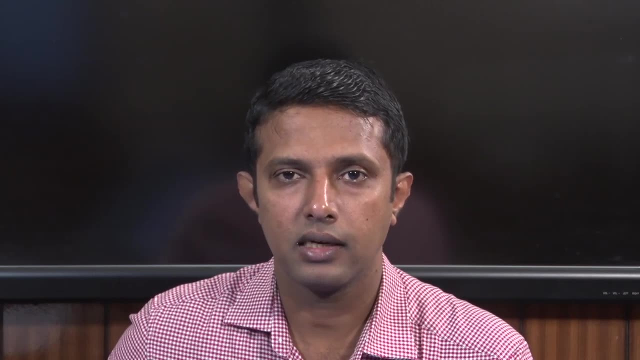 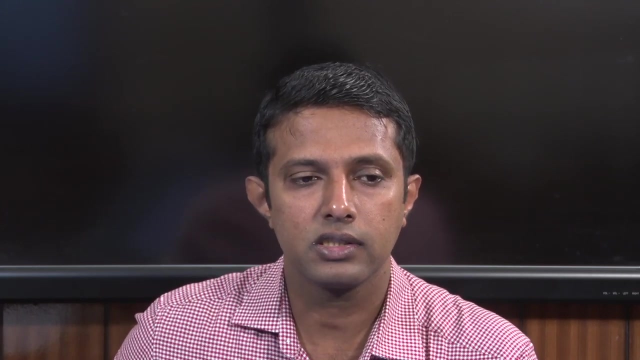 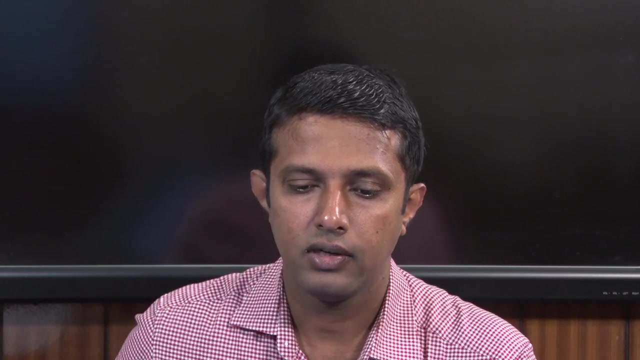 graph as well. When the graph is disconnected, what we can do is we can start a BFS at some arbitrary node in each connected component. Okay, Or we might need to discover what are the connected components, or we could just start BFS at every vertex of the graph. to start BFS at every vertex of graph. 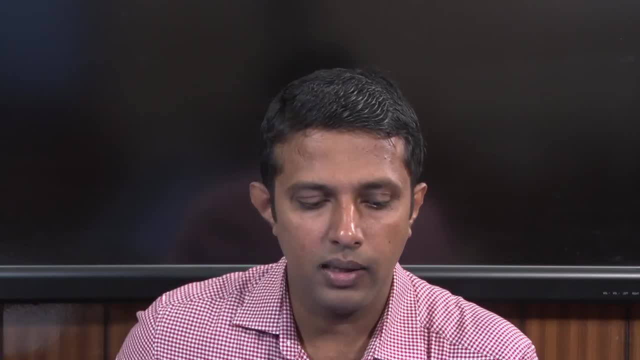 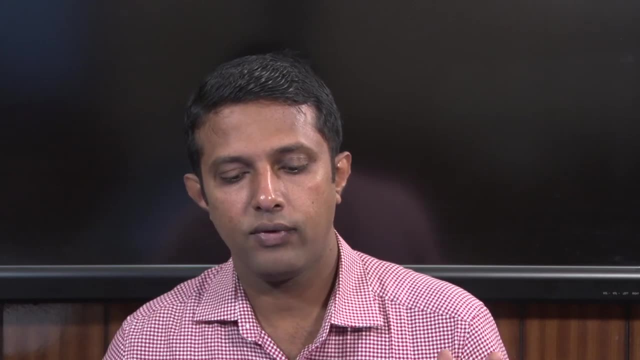 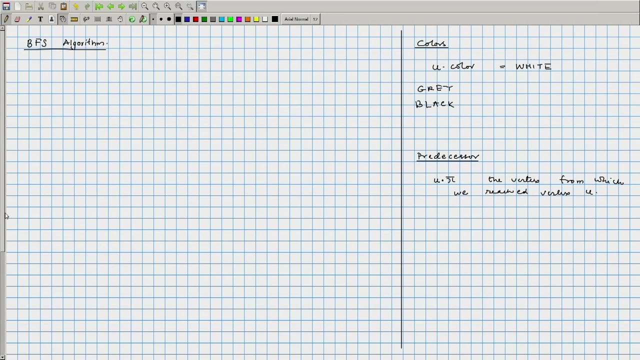 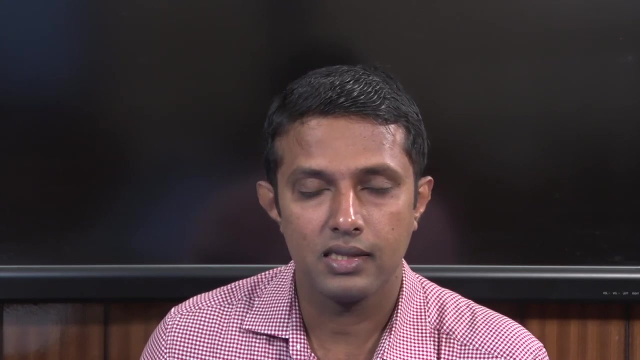 We need to check whether a certain vertex has already been covered by any of the previous BFS. So while doing the breadth first search, if we have already seen some vertex as part of searching certain other component, We can ignore that BFS search So that modification can be made and directed graphs. essentially, the same algorithm would. 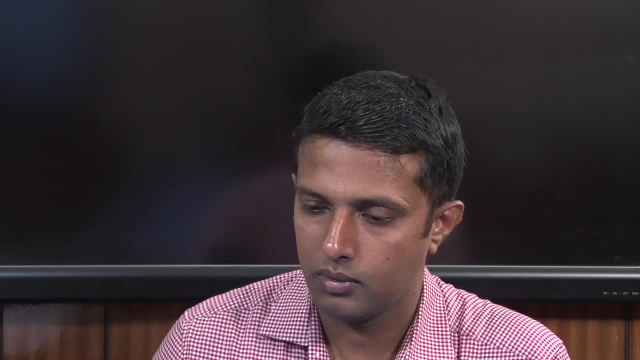 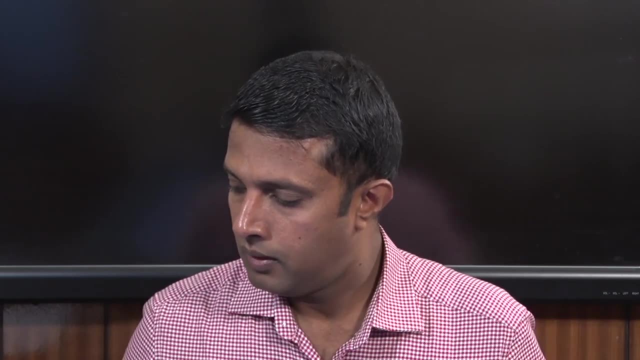 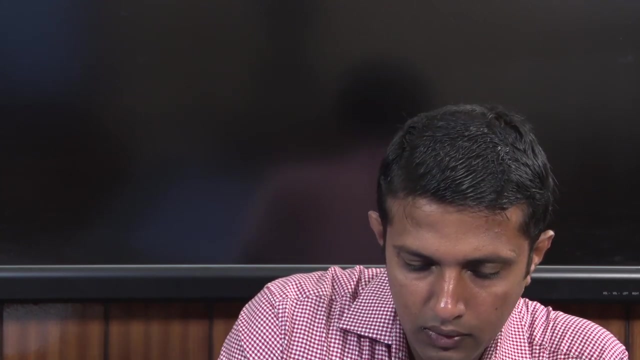 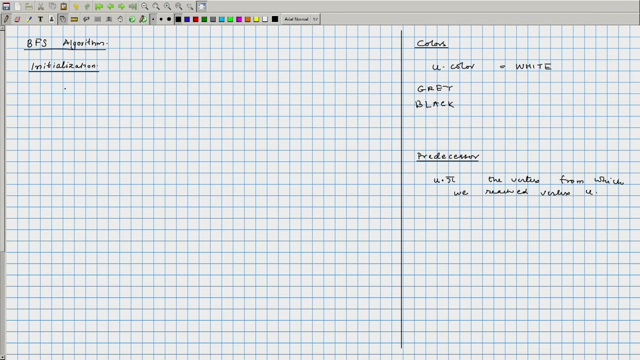 work. But for simplification, just to keep things simple, we will just look at the undirected example. Okay, So in the BFS algorithm we have to initialize the colors. Okay, Okay, Okay, So there is an initialization phase wherein for every vertex, so u dot color will be set. 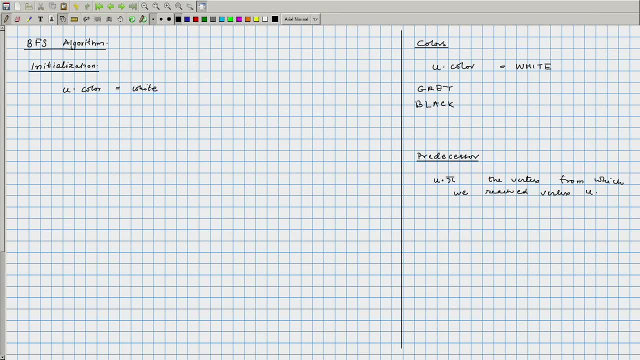 to white. That means at the start, vertices are all unexplored. So we will assume that the BFS algorithm, which we may call it as BFS. It has two parameters: the given graph and the starting vertex s. Okay, And for every vertex, the parent u dot pi will be equal to nil. 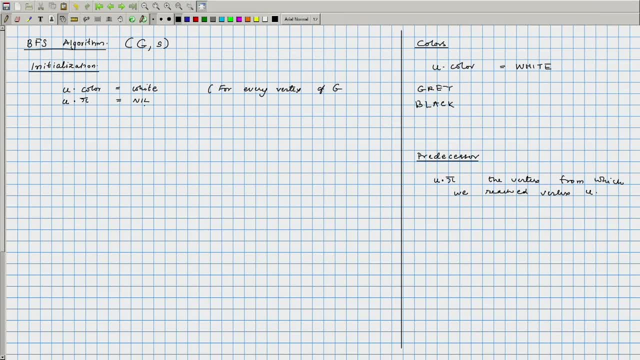 So initially we do not know what is the predecessor or parent of a particular vertex, So we will just set it to pi As our algorithm progresses when a node is discovered for the very first time, the node, the edge which caused the discovery of this particular node, 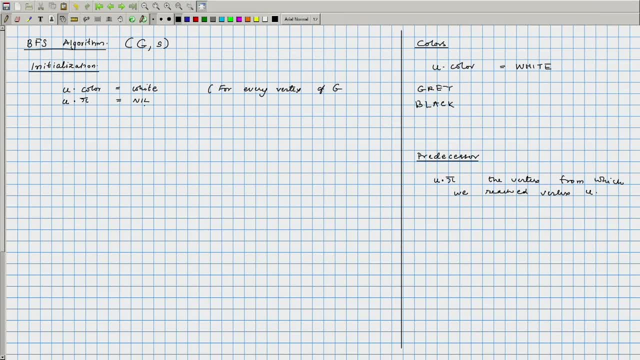 The node will be explored and that edge will tell us what is the predecessor of the particular node that we have just now found. Okay, So initially this is set to nil, And then we can also initialize the q. we will call it as a the q, we will name it as q itself. 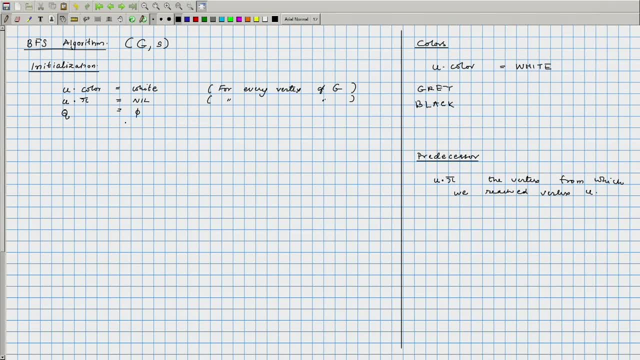 and this is set to empty. Okay, So there is an empty q. The q will be used to track the vertices and it is initialized to empty. Okay. And then what the algorithm does is: it will repeatedly explore for whatever is there in the q. 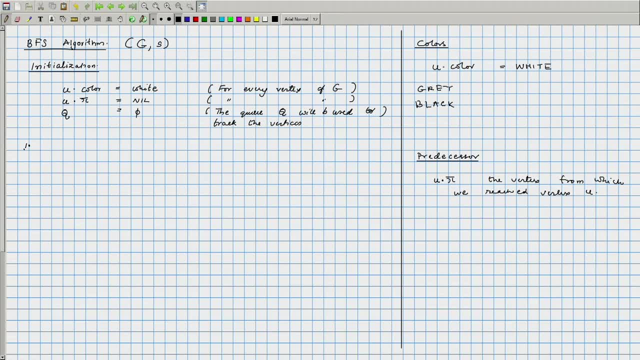 Okay, So after the q has been initialized, we have to add one element. So we will add s to q, The starting element that we had, the starting vertex that is added to the q, will be the first step of the algorithm, And then 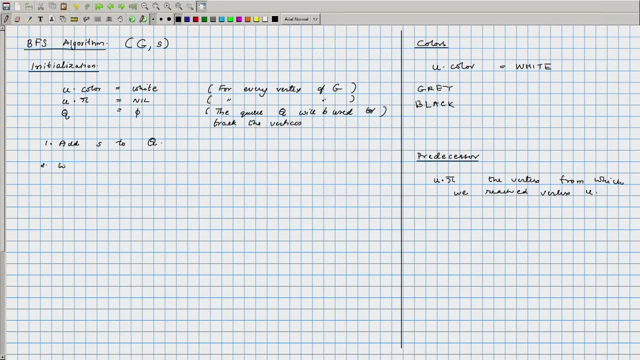 While Okay. So Okay, While q is nonempty, we will repeatedly do certain actions, So delete an element from the q, So we will call this deleted element as v from q. So q is a first in, first out data structure, which means the element that you have added. 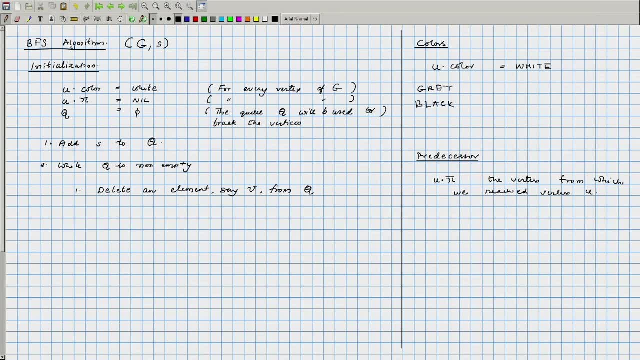 they will be removed in the same order. So at the start we have added just one element. So when you try to delete, the first element that will be deleted is going to be s, and then for every neighbor of v. So we have deleted one particular element. 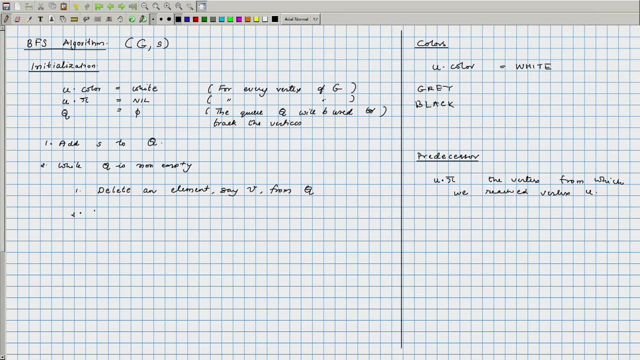 For each of its neighbors. we would, we would start exploring those vertices. So for every neighbor, let us say u of v. we will do the following: So we have one particular node that is deleted and that might have many neighbors, and for each of the neighbor, if it is an unexplored neighbor. 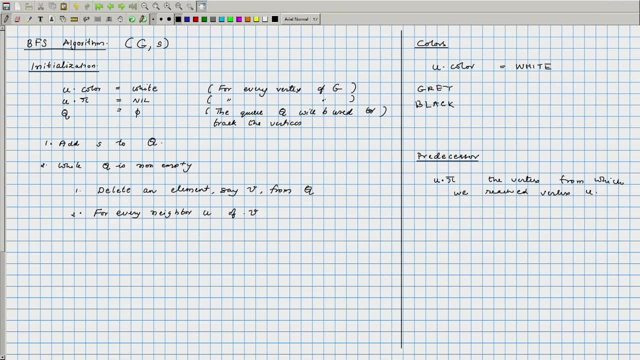 Okay, Okay. So, even though I mean, this vertex has not been explored before, we would want to do something with it. If it has already been explored, we will just leave it as it is. So if u dot color is equal to white, in that case what we will have to do is we will have 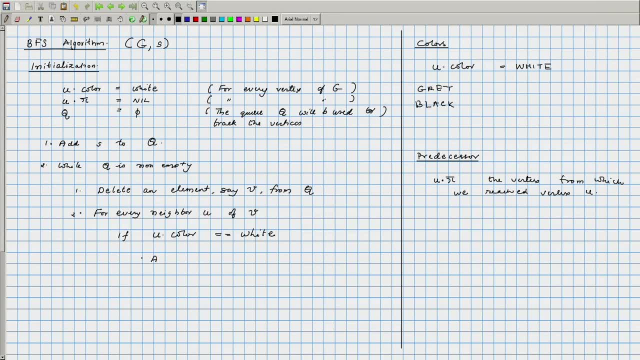 to push this into the q. and before adding it into the q, we will change its color. So this means we need to process it. so we will change its color and it is. the processing has begun. u dot color is equal to gray. Okay, And its parent. u dot predecessor this: we will set it to v because v was the vertex from. 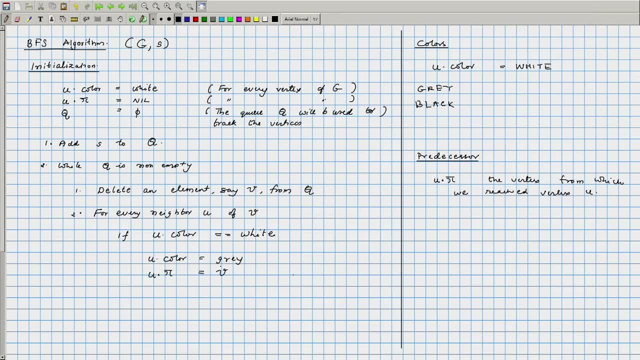 which we visited u because u is a neighbor of v. Okay, So the parent is being set, And then we can add u to the q. Add u to the q- Okay, Add u to q. And after this processing is done for every neighbor, we can change the color of the vertex. 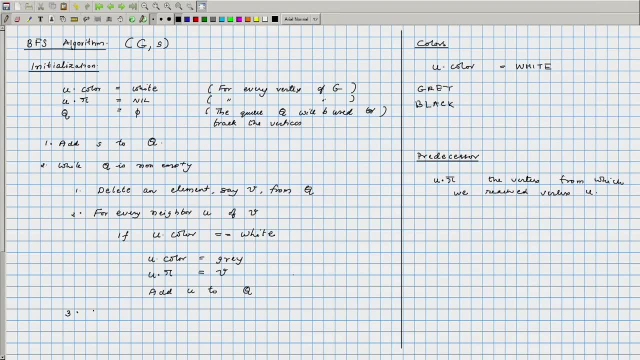 v to black, because v has been processed, So v dot color is equal to black. Okay, So that is the algorithm. So now let us see this in Action. So let us say, we have this following graph: Okay, Okay, Okay. 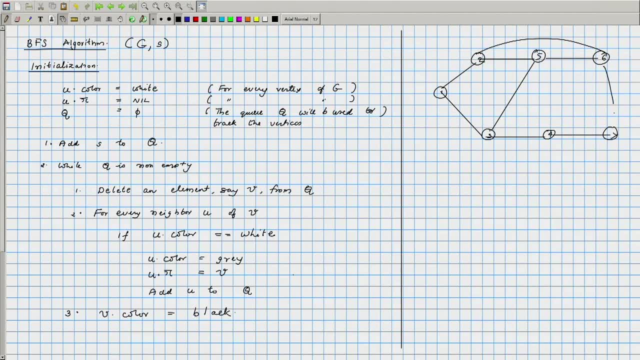 If, if you start at vertex 1, so this, we will just maintain a Q. so this is our initial Q and we will first add vertex 1 to the Q. that is the only element that is there in the Q, ok, and then we delete 1,. so initially, the color of all vertices are essentially 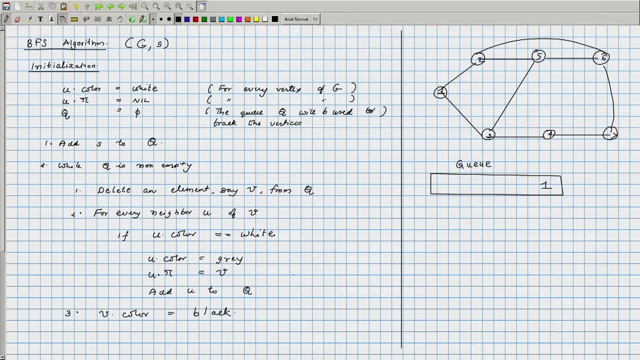 white. ok, once we have added, the color of that vertex changes. it becomes grey. So 1 is now a grey vertex and we will look at all the neighbors of U and change its color and we will set its parent to 1.. So the vertex 1 has 2 neighbors, namely 2 and 3. ok, so 2 and 3. their color is being changed. 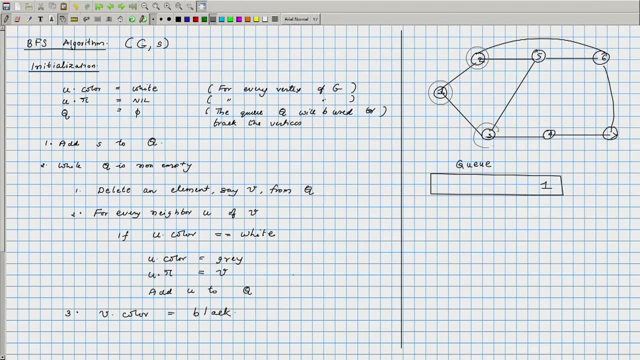 to grey, Ok, And the parent is being set to vertex 1,, so there is going to be so by this arrow I will indicate the parent. so 2's parent is 1,, 3's parent is also 1, ok, and after this means: 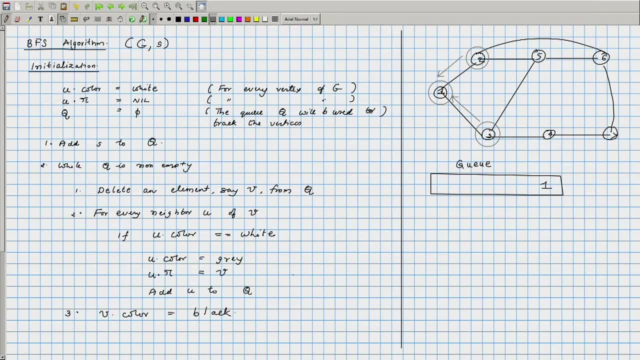 so this is the step that you do, and 2 and 3 has been added. So we may assume that first 2 is added and, after the processing is done, 3 is added. Ok, So vertex 2 would be added and vertex 3 would be added and we would have taken off 1 after. 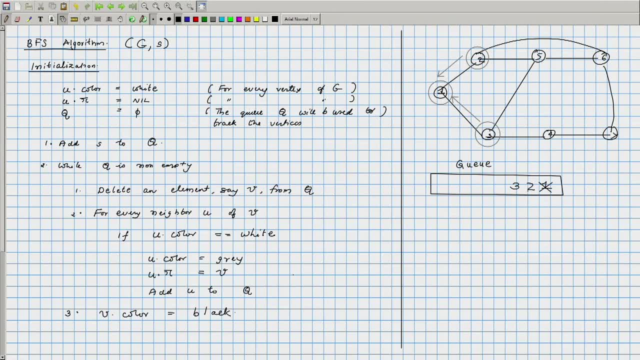 this. ok, so that would have been the first step. we have deleted that element and we have changed the color of 1 to black. ok, so now it is no longer grey, but it has become black, indicating The full processing is over. The queue is still not empty, so we will pick out vertex 2: ok. 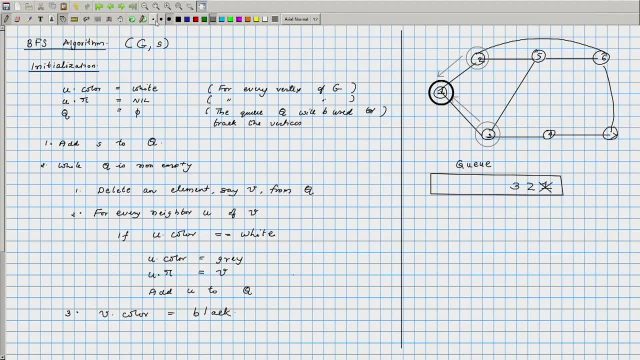 And if you look at vertex 2, that has been deleted. once vertex 2 has been deleted, we will look at all its neighbors. Vertex 2 has, namely, 3 neighbors: 1,, 3 and 3.. Ok, Ok, And 5, sorry. 1,, 5 and 6 are the neighbors ok. 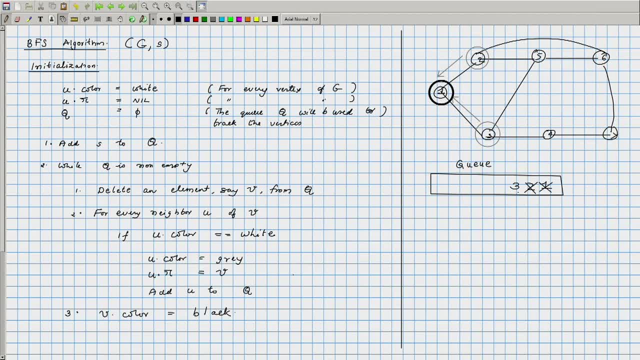 When you look at these neighbors 5 and 6, both are currently of color white, so we can add them ok. So let us say we first add 5 and then add 6, ok, so that goes inside the queue and their color, as well as parent, is reset. 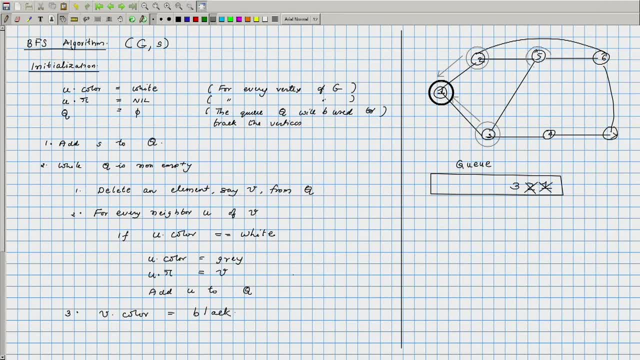 So 5 becomes the first neighbor. let us say it is 5. ok, so color is changed and the parent is set to and 5 is added. and after 5 is added, the next neighbor of 2 is going to be 6, that. 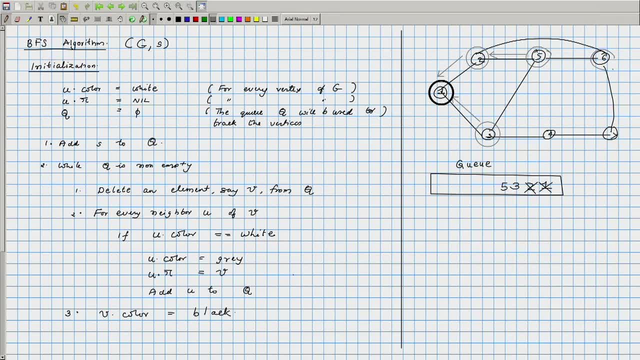 is also going to change its color to grey, Ok, Ok, And we have a parent for 6, which is 2, and 6 is been added into the queue, ok. So, after 5 and 6 is been added, the next node that you process is 3,. 3 has again 3 neighbors. 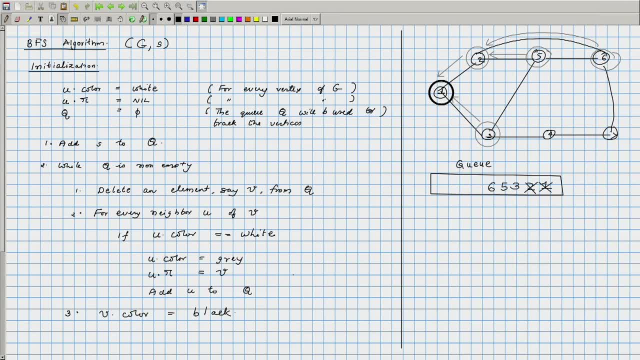 1,, 5 and 4,. out of them, the only white neighbor is going to be 4, so that will be converted into grey and the parent would be set to 3.. And additionally, we would have 4 coming into the queue and 3 by the stage is done with. 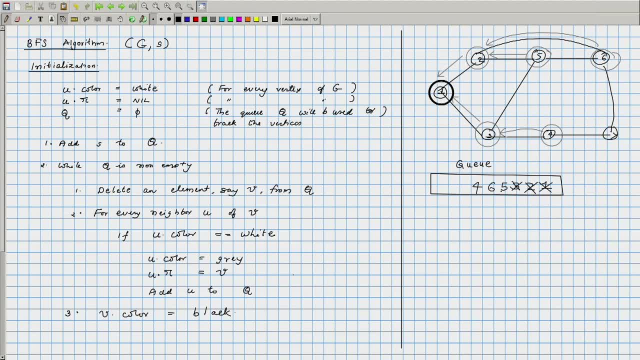 ok, we would have deleted 3.. The next element that is going to be deleted is 5,, but there is no further processing to be done with 5., 5., 5., 5., 5., 5. 5.. 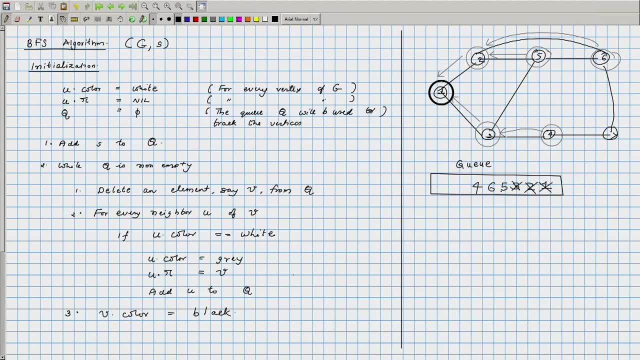 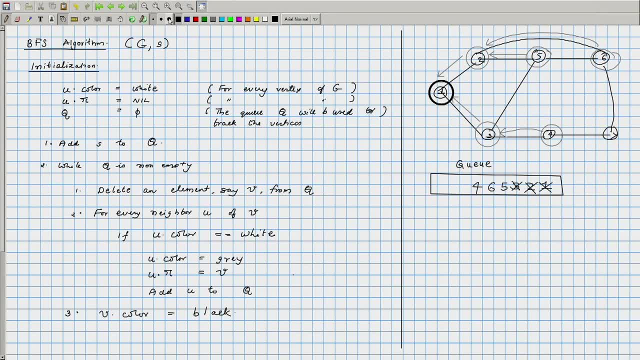 we would have changed the color to black. So there we skipped couple of steps. we would have changed 2 to black and 3 to black after that, and then 5 to black. Ok, Ok, The next node that is going to be processed is going to be 6,. 6 is one neighbor, namely. 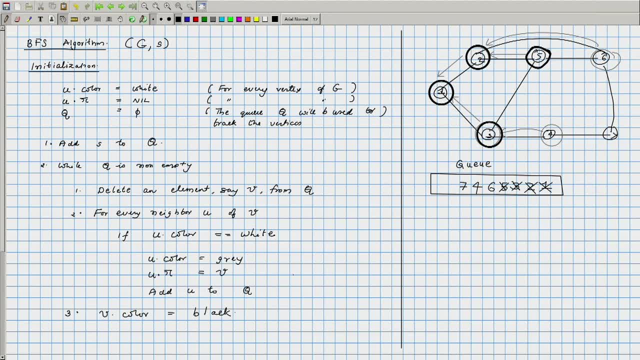 7, so we will add 7 into the mix, into the queue, and its colors are changed and the parent is also set 6, the other neighbors of 6 are 5 and 2, which surely cannot be added, and after 7 has been added we can say that the processing of 6 is over and its color becomes black. 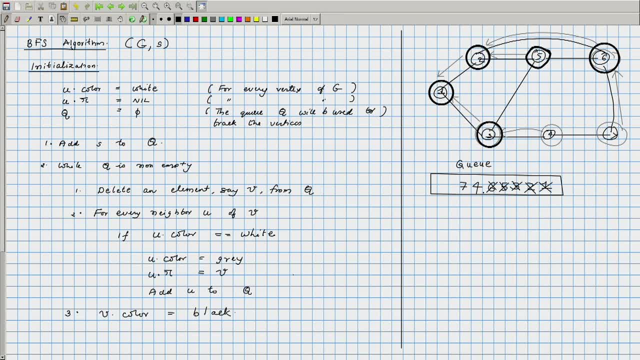 The next node that would be processed is 6.. Okay, 4, 4 has 2 neighbors- 3 and 7, but both of them have colors different from white and therefore there is nothing to be done with any of the neighbors of 4, 4's color will. 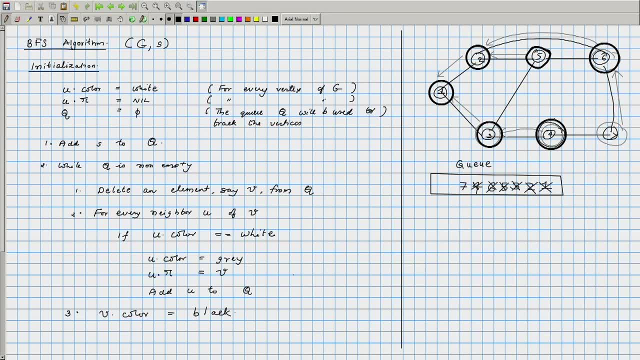 be changed to black, and then the queue contains only 7. that is removed. all the neighbors of 7, namely 6 and 4, has already been processed, So they are black in color and therefore nothing has to be done with 7 other than change. 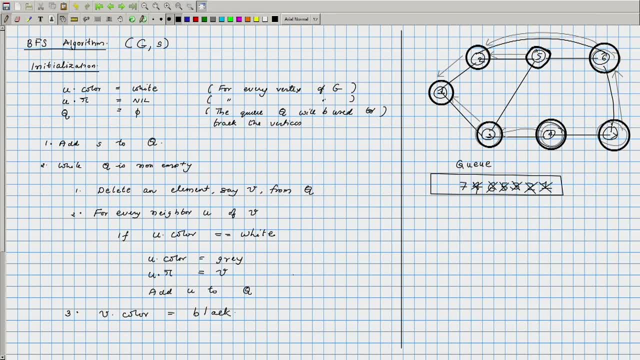 its color to black. okay, and at this stage the queue is again empty, so that processing is over and we would have traversed all the nodes by that. okay, Note that if you look at just the predecessors of each node, that will be an interesting diagram. 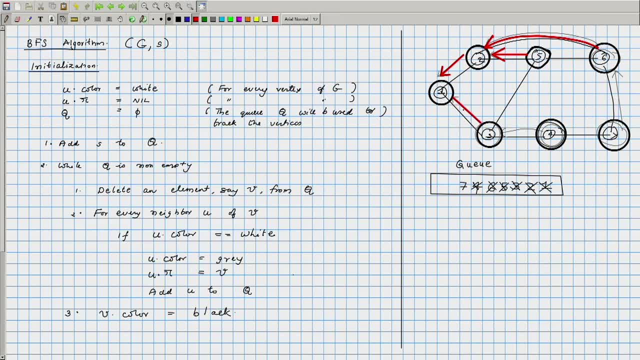 this will be a tree. There will be no cycles. it is a directed tree, with every node having a unique path to the vertex 1,. okay, and so that tree is called as the VFS tree. okay, and this entire algorithm can be implemented in linear time if you maintain the initial graph as an adjacency. 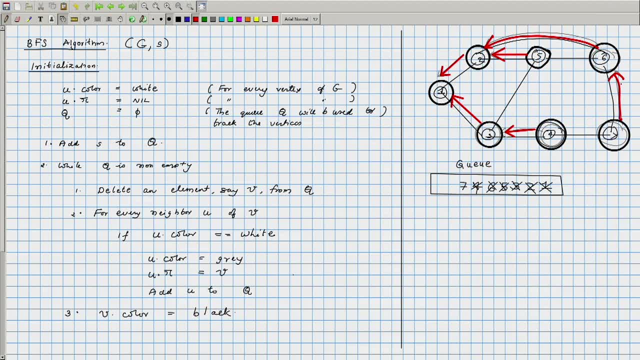 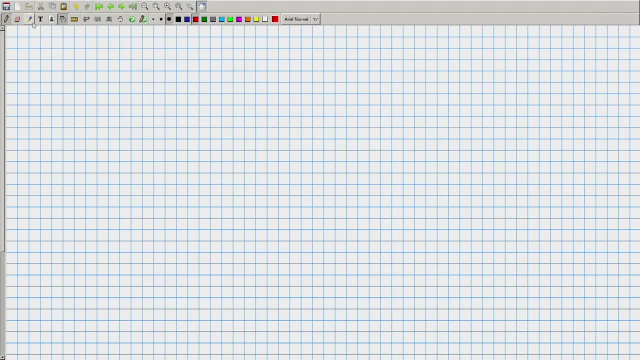 list. okay, Okay, 3.5.. So the search algorithm that we will see is the DFS search. so let us begin the DFS search, or the depth first search. so, again, we will have two parameters associated with each node, namely its color and the parent. okay, 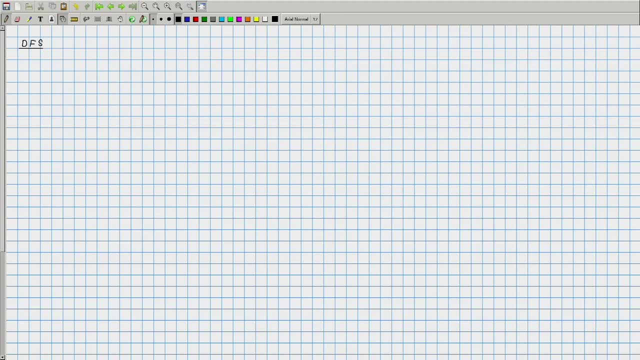 Instead of using a queue, we could implement DFS search- Okay. DFS algorithm using a stack. we will see a recursive version of the DFS algorithm wherein we will not have to explicitly maintain the stack. the recursion would essentially keep track of the stack, okay. 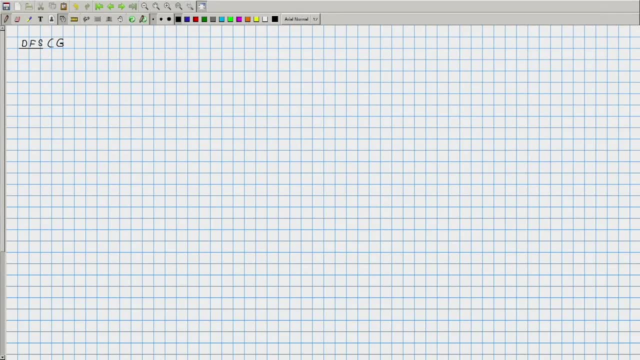 So DFS algorithm. this will require two inputs, two parameters. one is a graph itself and the other is the starting vertex. We will have an initialization phase, Okay, Okay, Okay, Okay, We will run subchar: 휴대. 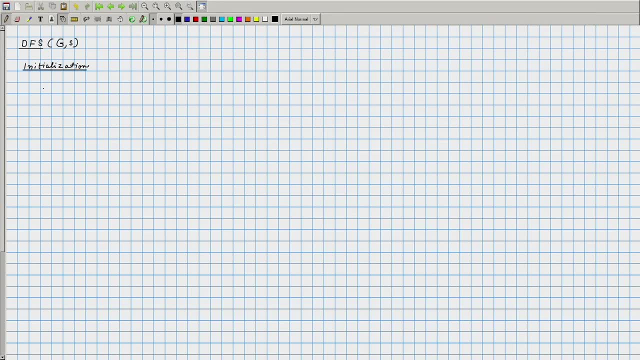 Okay, So we are going to look at the DFS algorithm. so, for example, here we just filled out the line EI1, EI1, so we have one operation like this. look at this: EI1, EI3 is in on the 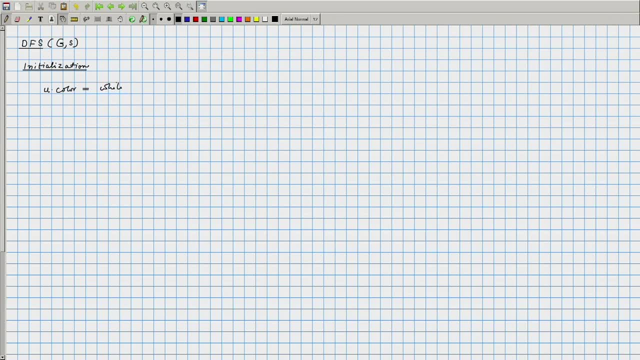 property inside the DFS能 지 적는 자 an excel to basically request the comma parameter in the World Security Law. ok, We will see a DFS algorithm on X, refugees or any meeting data save values from here. Okay, Okay, particulargraph, we need to do this. initialization ok, and once this is initialized we can call. 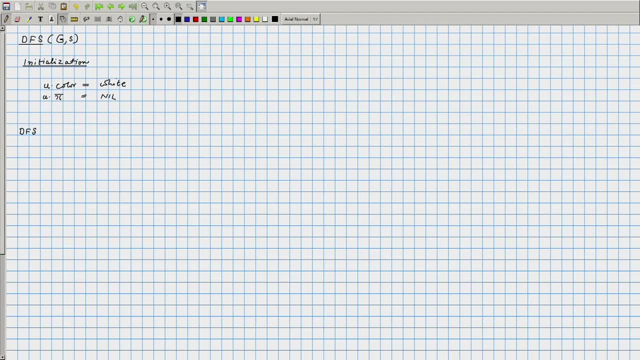 our DFS routine. So write down the DFS routine. two parameters: g and s. we will assume that the initialization has already been done and what we will do is the following: So we will make the colour of s to be grey, So s dot colour is equal. 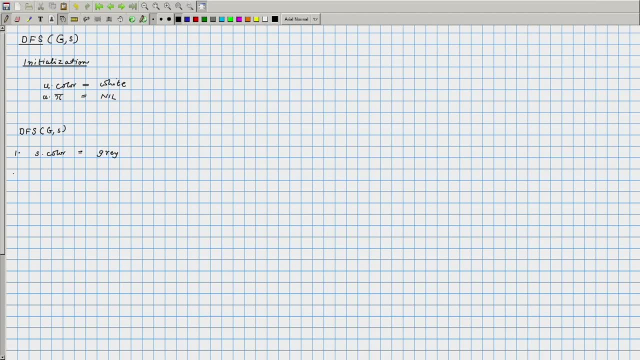 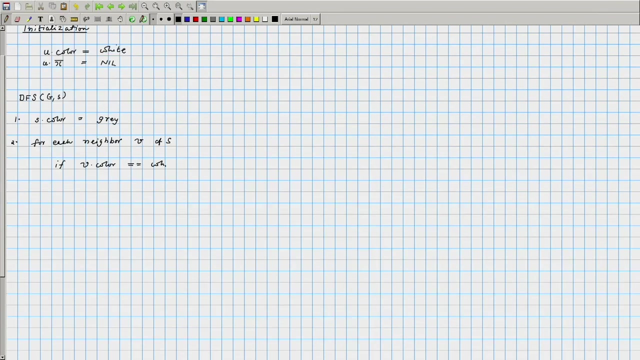 to grey and then for every neighbour of s for each, we will do the following: If v dot, colour s is equal to white. So while the DFS is being run, each vertex it is colour could change. we want to ensure that the colours change from white to grey to black. So if you have 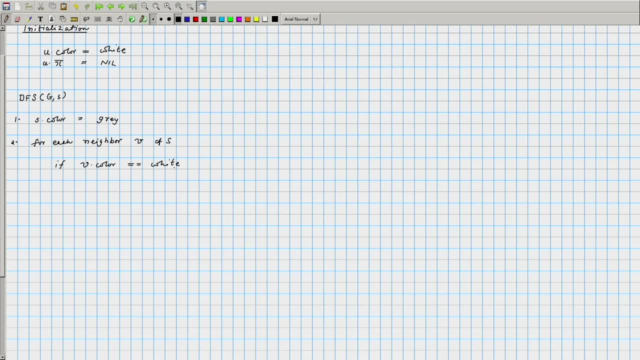 a white coloured vertex. that means it is not been explored yet and therefore we are ready to explore it now, because it is a neighbour of vertex s, and what we will do is we will write down the initialization, So we will assume that the initialization has already. 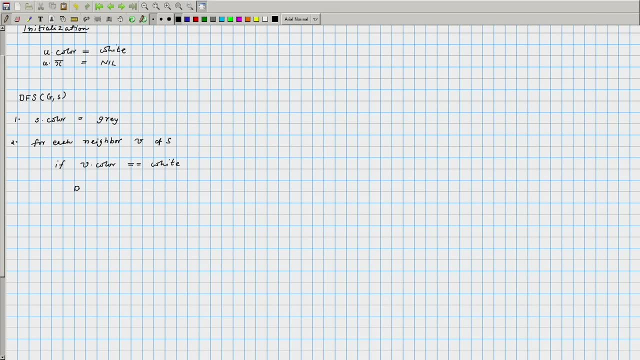 been done and once this is completed, we will just call DFS. with this new vertex on the same graph, So DFS g, v and after all the vertices of s has been processed, we can set the colour of s to black. s dot colour is equal to black. ok, Maybe it is at this point just. 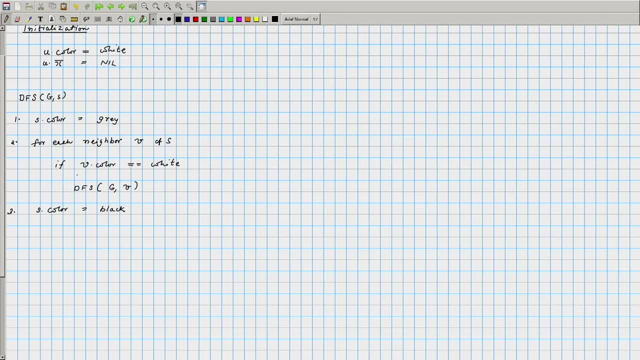 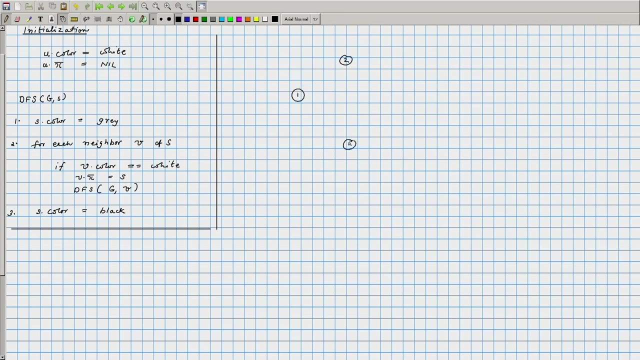 before calling DFS, we will need to set the parent. V dot pi is equal to S, so let us see how this works. ok, So suppose we have this particular graph And we start DFS at 1. ok, So initially every vertex is of color white and the parents there are no parents, everything. 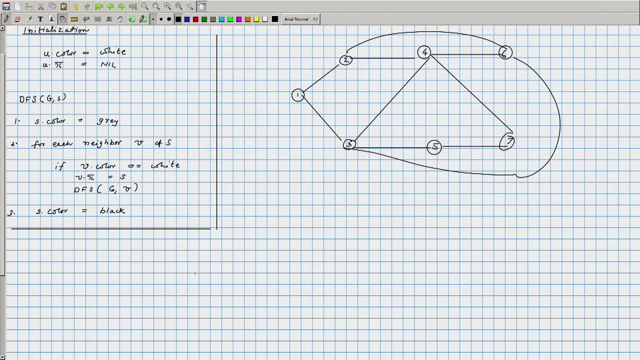 is nil ok, and when you call DFS on vertex 1, what happens is the color of that vertex immediately changes to grey, and then what happens is the recursive calls start. So for every neighbor, the vertex 1 has 2 neighbors, Namely 2 and 3. for each of them we are going to call the DFS. 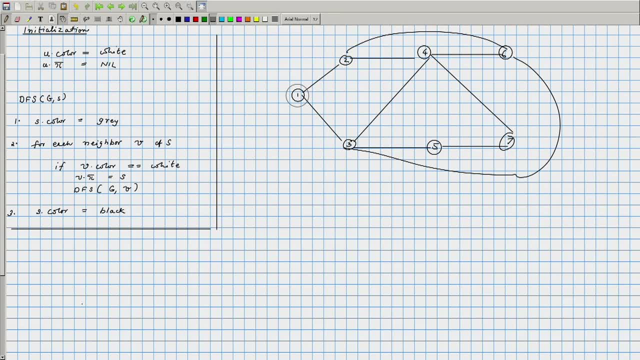 Let us assume that the first DFS call will be for 2 and the next DFS call will be for 3.. But before that we need to check whether those are white. indeed, they are white and therefore we can make those calls. ok. The very first call that will be for is DFS 2.. 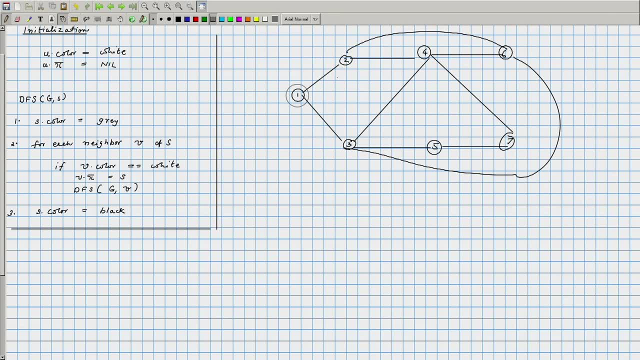 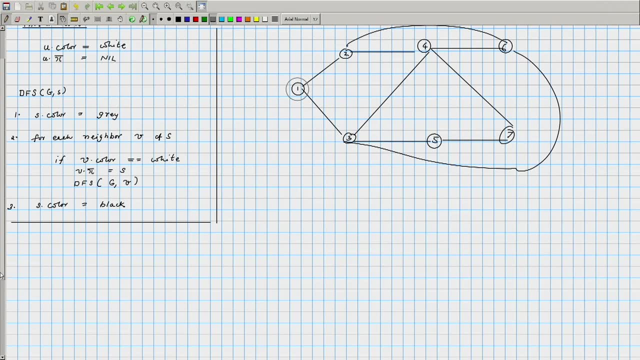 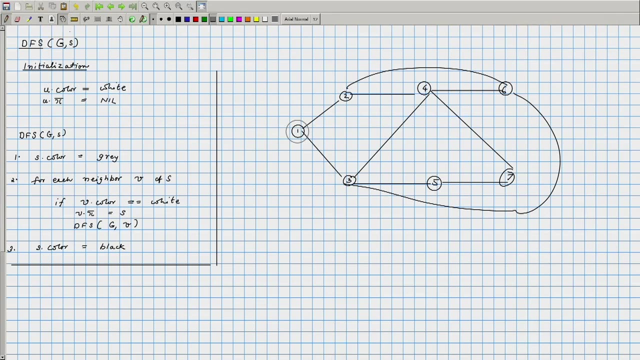 When DFS 2 is being called, what happens is it will go into the recursive call, the recursive routine, Ok, And inside that the color of this would be made grey, ok, and we would have set the parent. ok, The parent of 2 is going to be 1, and now we are going to process DFS g with 2.. 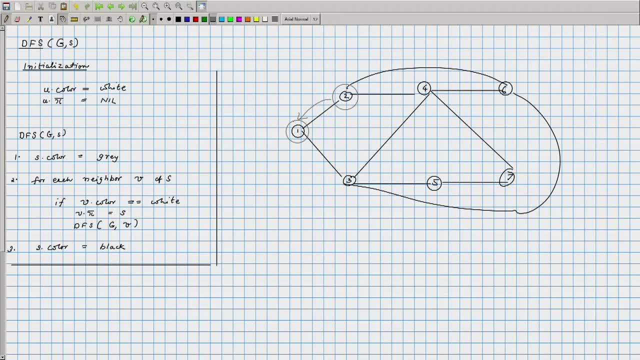 When we are running the DFS on 2.. Its color would have been set Set to grey and then for each neighbor of 2, we will have to process this particular code. When we will have to process these code segment for every neighbor of 2,. 2 has 3 neighbors. 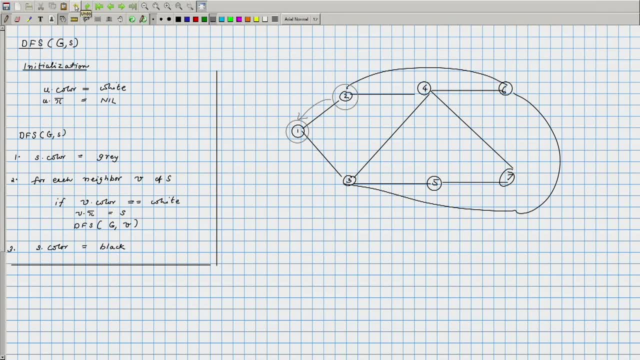 namely 1, 4 and 6.. But out of them, only 4 and 6 are white and therefore those alone will be processed. ok, So let us say vertex 4 is going to be processed First, so its parent is going to be set to 2, and while DFS g 4 is being processed, this: 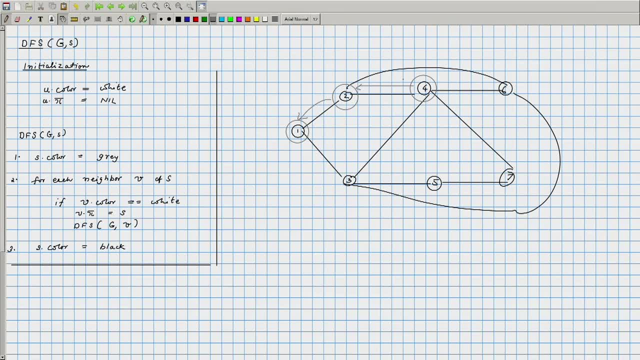 will turn into a grey node. Once this is a grey node, we will have to explore all its neighbors. It has 4 neighbors: 2,, 3, 6 and 7.. The white neighbors? there are 3 of them: 3,, 6 and 7. so presumably all of them will essentially 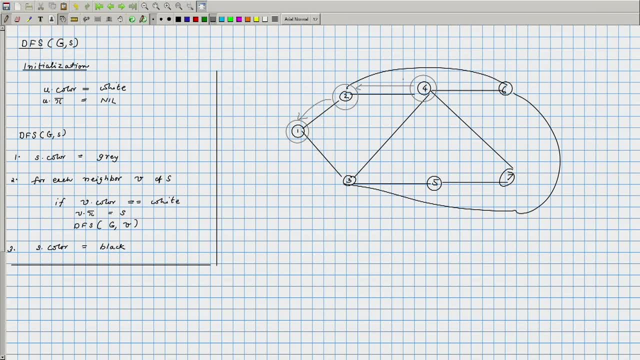 be processed. Let us say DFS 4, when it is being called the neighbor that is picked is that is picked first. is vertex number 7 ok, and therefore the parent would be set and 7 would turn grey and DFS 7 is going to be processed and DFS 7 is processed. 7 has 2 neighbors, namely 4. 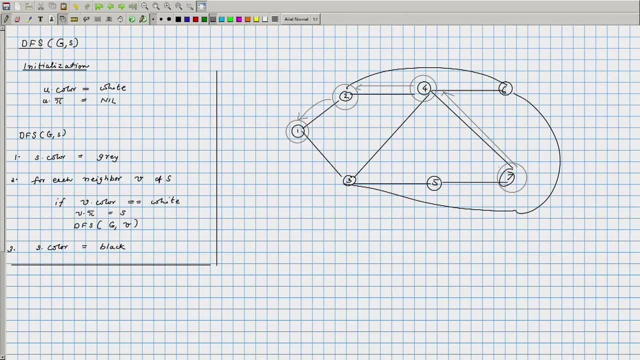 and 5.. The only white neighbor is going to be 5, so there is going to be a DFS 5, ok, and the parent is going to be set and DFS 5, it will look at all its neighbors. Its neighbors are 3 and 7 and 3 is still white in color. so that would be processed and that 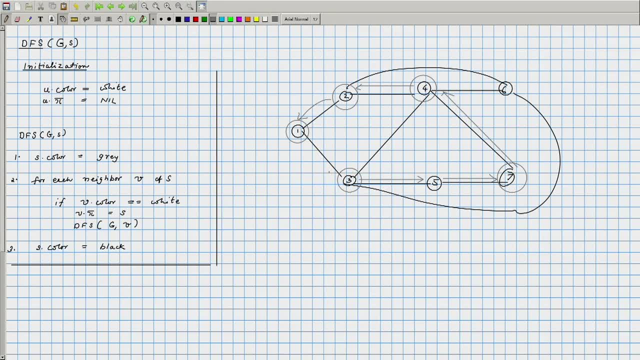 turns grey and when you are processing 3.. This becomes black. this would have become black and the call returns back to 2,. 2 has one more neighbor to be processed. 8 after 8, processing is done, this becomes black, and then 2 becomes black and then 1 becomes black. ok,